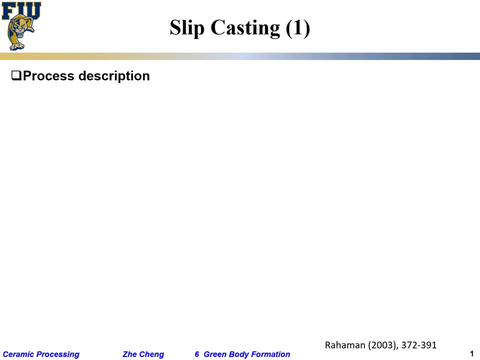 So slip casting the process description. Essentially, you have mold, quite often porous mold. You pour the slurry, your suspension into it and over time, by suction action, you apply vacuum or just by itself, the capillary suction, the moisture goes away and then you have so-called slip casting. 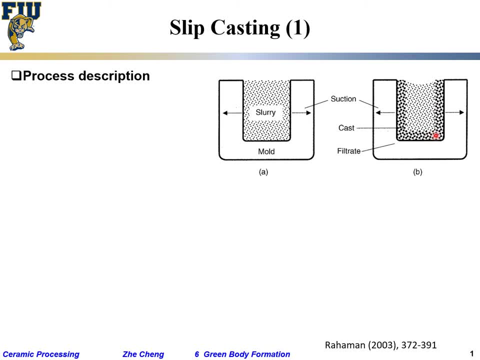 The powder cast, wind cast, the powder compact. okay, Slurry is poured into porous mold which sucks solvent away by capillary force. Of course you can apply vacuum. it's more expensive, but if you have to do it, you do it Generally slip casting mechanism, this so-called law. of course we are not so much into it. The solvent flux: we define the flux J as K over. 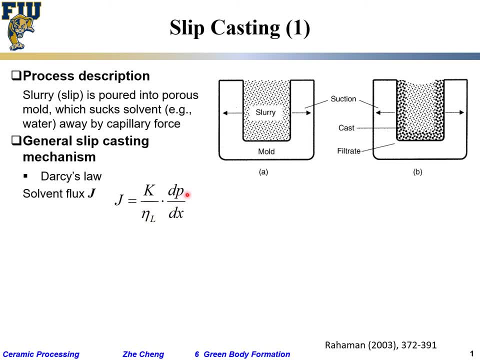 this eta and the dp over dx And the K is permeability of the porous medium, your mold, porous mold as well as your already deposited or consolidated layer. You see what I mean. This part, the already kind of like partially sedimented portion, will not be very dense. It still allows. 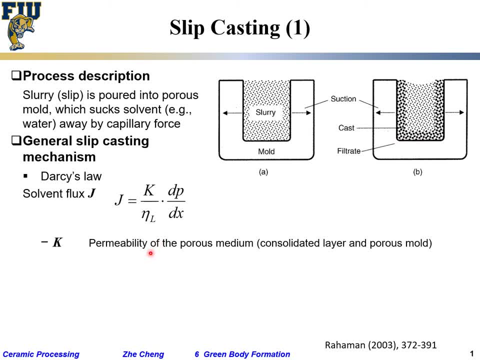 the solvent to go away. Permeability of this cast, as well as the mold And then this eta for solvent viscosity and the dp over dx pressure gradient between inside and outside. Of course, the higher the permeability, the higher the solvent flux. 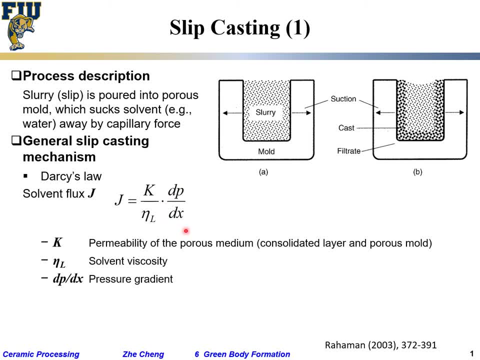 The higher the so-called pressure gradient. how fast does the pressure decrease from one side to the other side? the higher the solvent removal rate, The higher the viscosity. higher eta, the lower the solvent removal rate. Common sense, right, Kind of okay, makes sense Then. 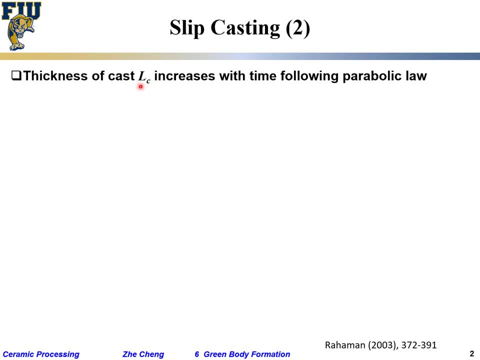 slip casting. Slip casting, So the density of your cast, of your solidified kind of solidified layer, increases with time, following like a diffusion parabolic relationship: L, your thickness for your cast. the square term equals a constant times, t, Or this one if we use diffusion as an analogy, like square. 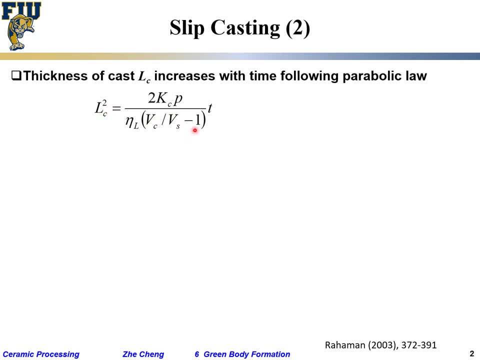 root of constant times, t, And at this constant we have still a number of so-called parameters, We have still the permeability of the already consolidated cast right. We are doing casting and the part that nears the wall first becomes packed higher density And that becomes a. 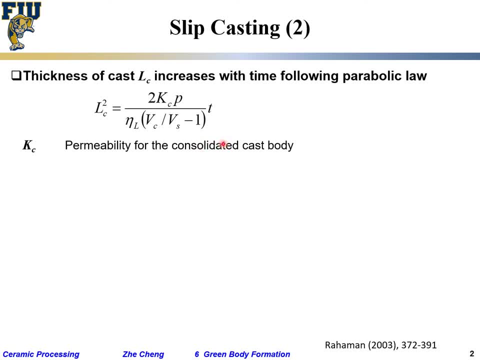 barrier layer for liquid tires. Okay, So in general nothing happens. All right, Thank you är for your continual solvent motion. So the permeability of that consolidated layer is also important in this case P pressure difference across the cast body. 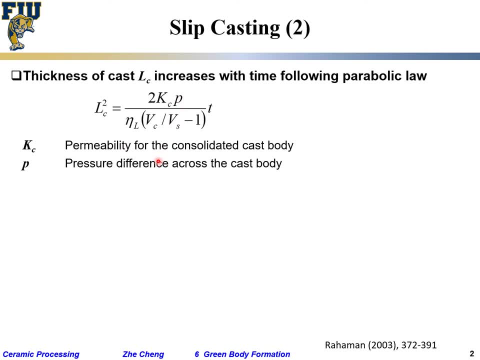 And, strictly speaking, I probably should use delta P. the pressure difference between the cast body inside, still liquid, versus outside And the viscosity and the volume fraction of the solid in the cast. Vc. volume fraction of solid in the cast body and volume fraction. 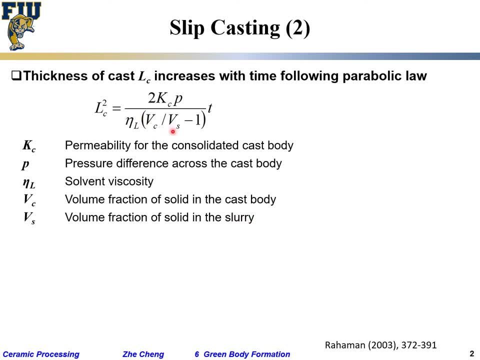 of solid in the slurry, this ratio. So it just gives you an idea of how fast would my cast thickness increase over time. It gives you an idea roughly how fast it is going to be And the implication would be the thickness growth rate. 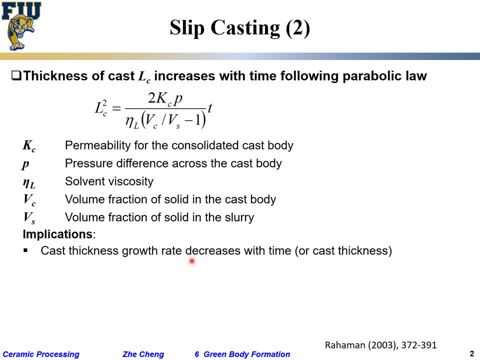 would decrease with time. How do you know it decrease? You can do differential or you can say: OK, this is following kind of parabolic diffusion, Like a diffusion: the longer the time, the slower your diffusion appears to be OK. 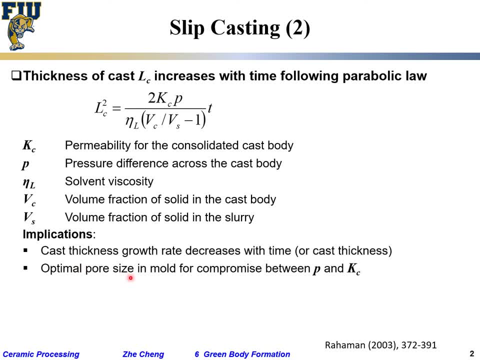 And optimize. Optimize pore size is a. you need an optimized pore size for compromise between pressure difference and permeability. If your pore size is too large, your permeability would be what? If the pore size is too large, which means you allow the liquid to go through? 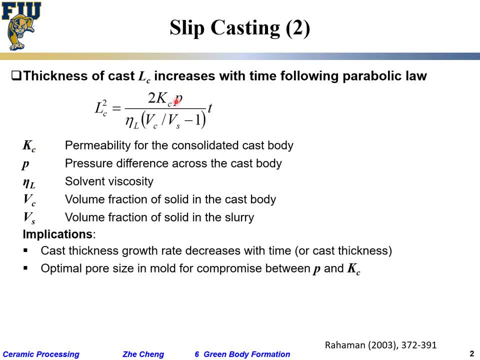 your permeability would be high, which helps, But at the same time, if the pore size is too high, you cannot maintain a big enough pressure difference Make sense. Remember: P is the pressure difference If the pore size is very large. you. 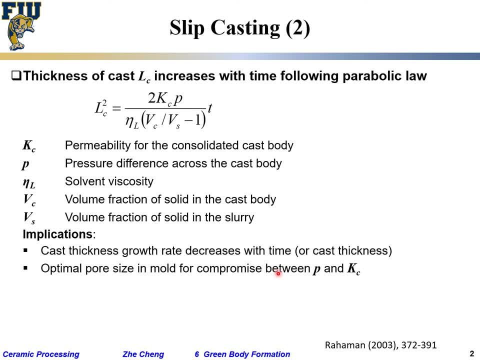 don't have a pressure difference. Extreme case: the same: It's open, completely open. You have no pressure difference. Make sense. So that's why we said OK, optimal pore size, not too large, not too small. If it's too small, no liquid can go through. extreme case: 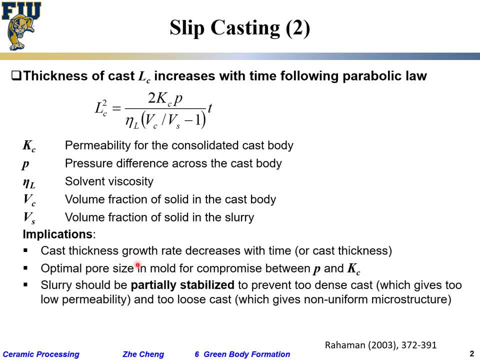 Right Permeability too small, Right Drops suffers And slurry should be so-called partially stabilized. We said, if it's too stable, the slurry is too stable. it's going to give us a so-called too dense cast. 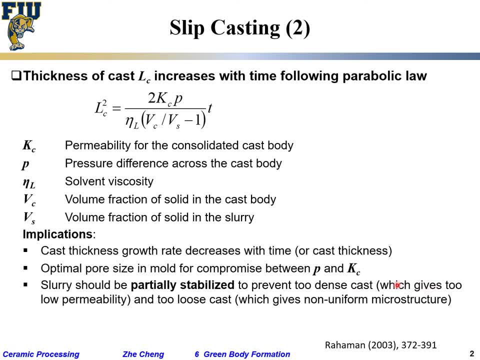 Too dense cast which gives too low permeability, which prevents further drying or removal of the solvent Make sense, Which means it does not work. That's what you want. On the other hand, you do not want your slurry to be completely unstable. 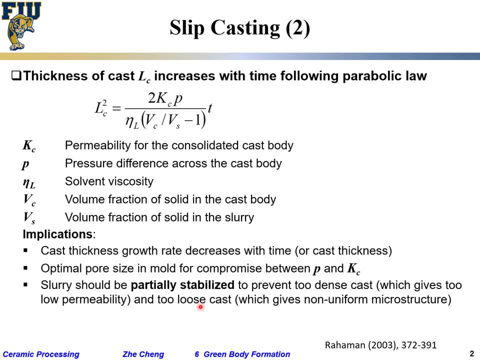 Otherwise it's packed too loosely, Everything loosely flocculated, and then it gives you too loose a cast green body, Make sense. So it's compromised. You see again, it's compromised, compromised, compromised. Intermediate condition, not too extreme. 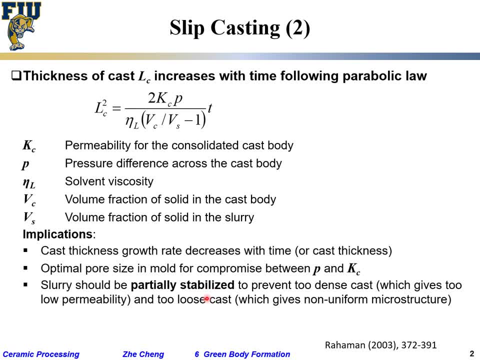 OK, We said Earlier you can try to stabilize your slurry or suspension by adding electrolytes, by adding polymer. But here we say you do not want your suspension to be too stable, Otherwise when they pack they give you.